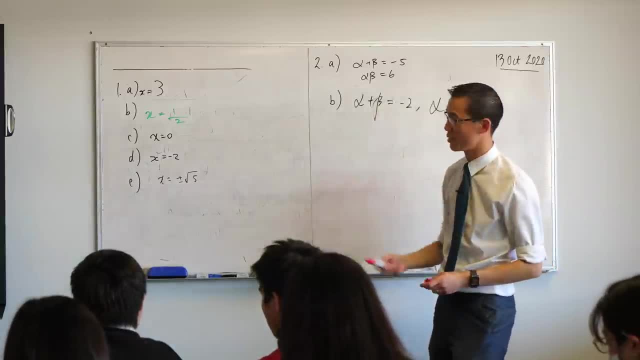 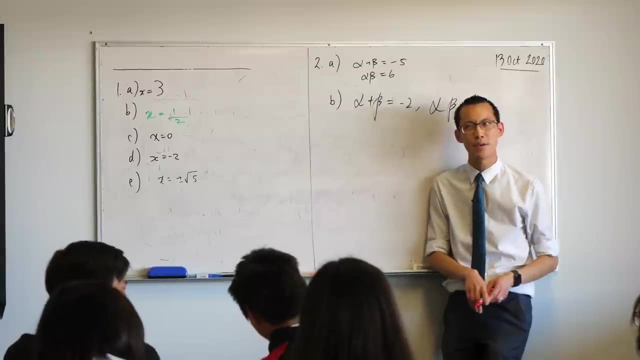 you've got another colour next to whatever colour, you just did these questions, pull that out and if you do not have another colour, borrow from someone and then fix that, because you'll find colours are going to be very, very useful in communicating and understanding what you're doing here. 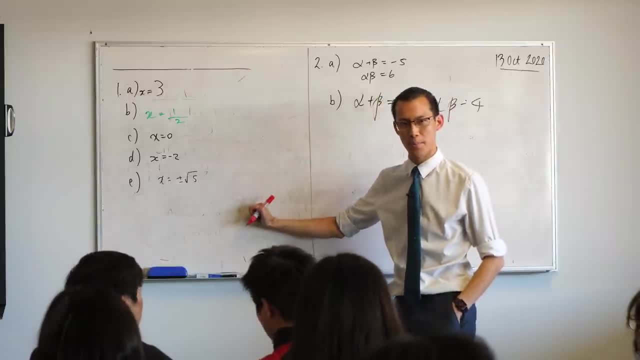 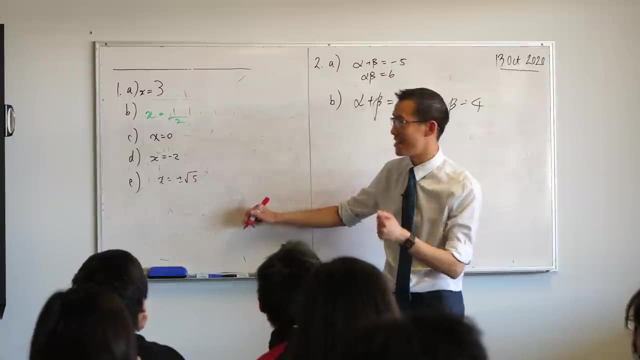 We went through a potted history of all the different kinds of numbers that we, as mathematicians, use all the time. right, and these are pretty familiar, right, the first number is the most basic kind of number that anyone has ever come up with, and I'm going to. 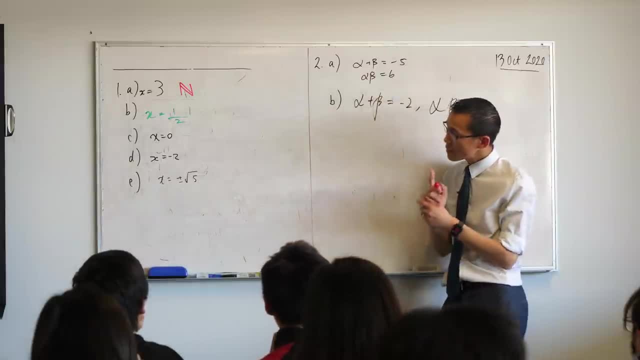 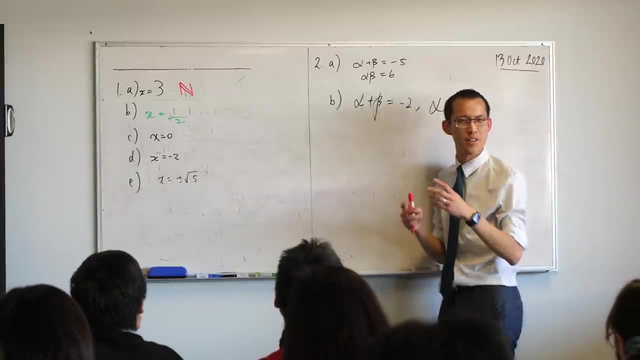 introduce some symbols here which you need to be aware of. This is an N. you can see it's got two sort of solid lines through it, which is part of set notation. when you see these two lines going through, you know this is not just a pronumeral, this stands for a whole set. 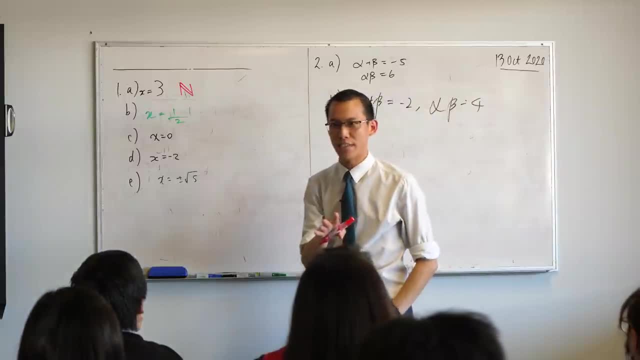 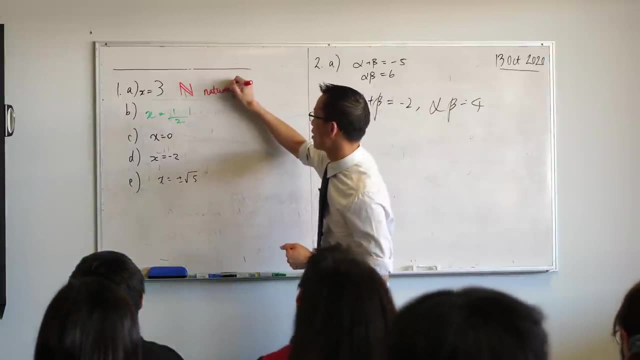 of different numerals This N stands for? does anyone have a guess? A very basic, important part of the number system, The natural numbers. very good, Also called the counting numbers, because that's exactly what we do with them: We count one. 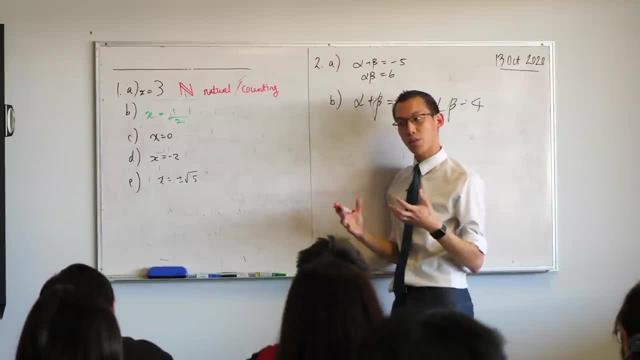 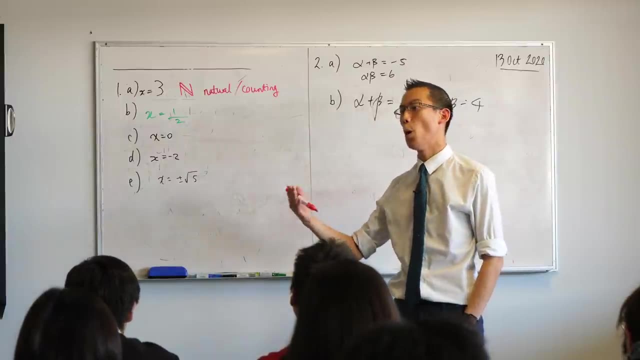 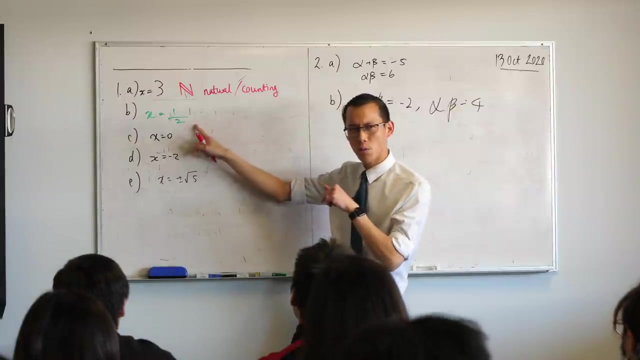 two, three, four Since pre-history, before things were written down, we were counting right, But fairly quickly we realised there are more numbers than just one, two, three, four and so on. These numbers here are not natural numbers, they're not counting numbers. you don't count up to a half. Does anyone know what? 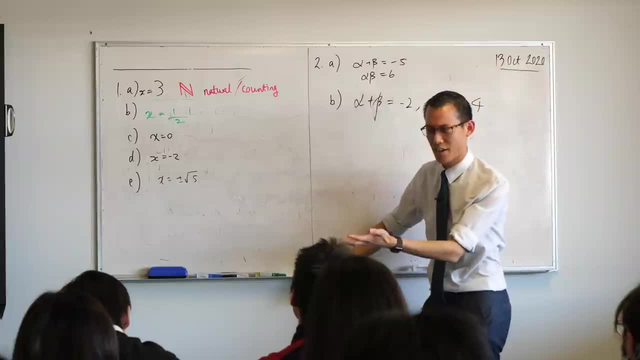 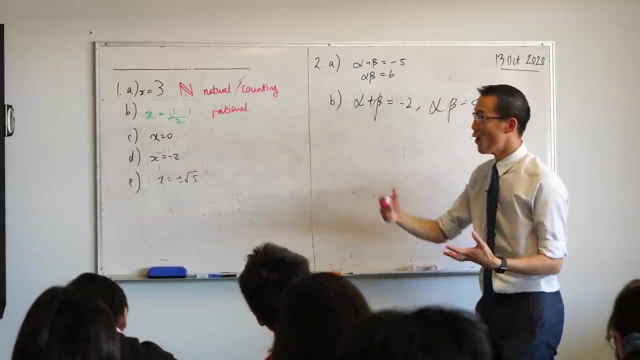 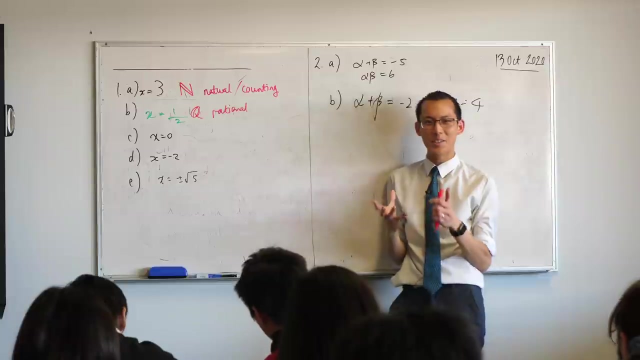 family of numbers. this belongs to Any takers. Yeah, go ahead. starts with an R, by the way. Rational numbers, very good. Now, because we like to try and be completely sensible. the symbol for rational numbers is is not an R, it's a Q. Does anyone want to guess? why? might it be Q? What word to do? 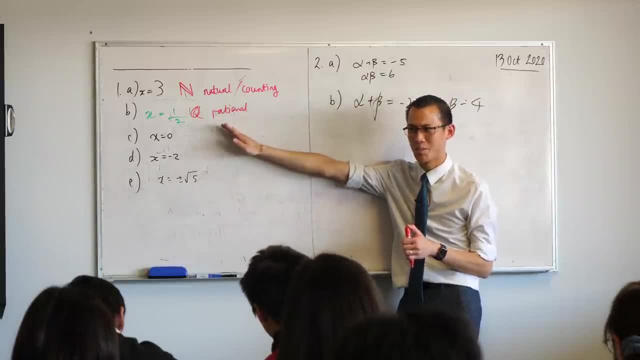 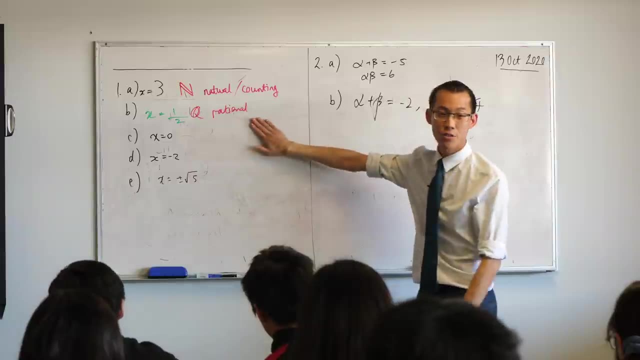 with this starts with a Q. This is division, right, Think, think, go ahead: Quotient: very good, So that Q is a reference to that idea. Rational numbers: again in the name it's about a ratio between two numbers, and so we're pretty. 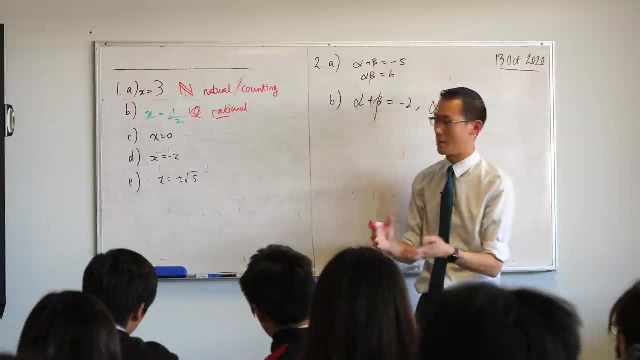 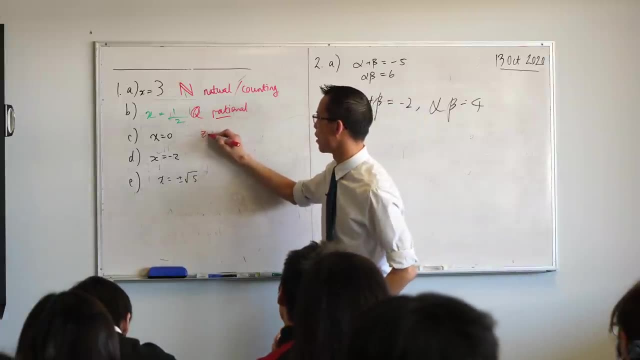 familiar with those, but they took a while to develop in terms of mathematics. Zero kind of sort of doesn't belong especially in to any particular family. but I do wonder, does anyone know how long did it take us to come up with the idea of zero? Does anyone know roughly when it came? 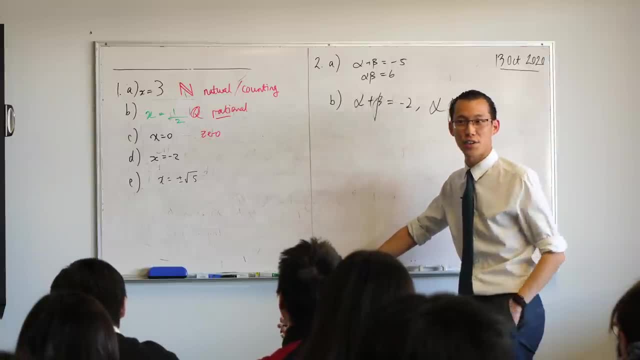 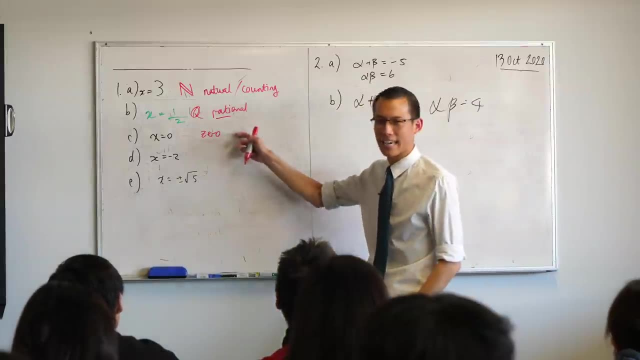 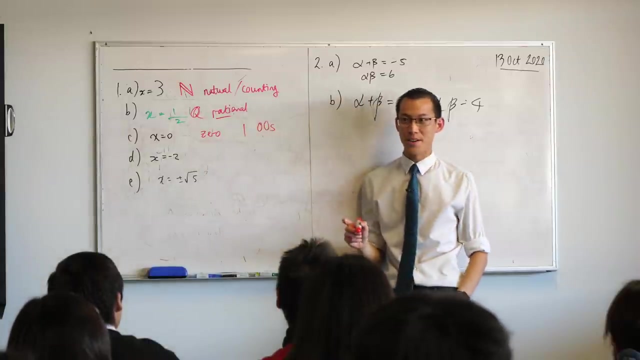 into vogue. I'll give you a clue: way later than you would think Any takers- Anyone- have. just hazard a guess: when do you think we really came up with this idea? Yeah, go ahead. 1900s, so it was a long time ago. longer than the 1900s, though, so we 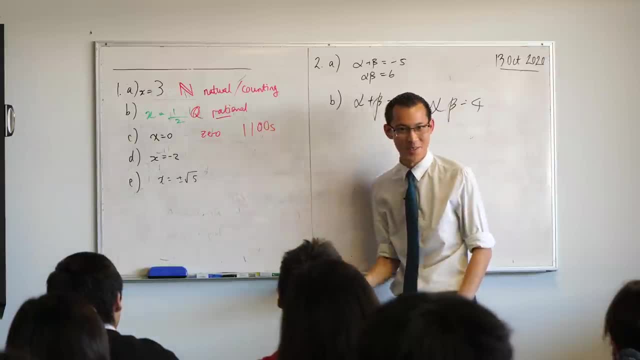 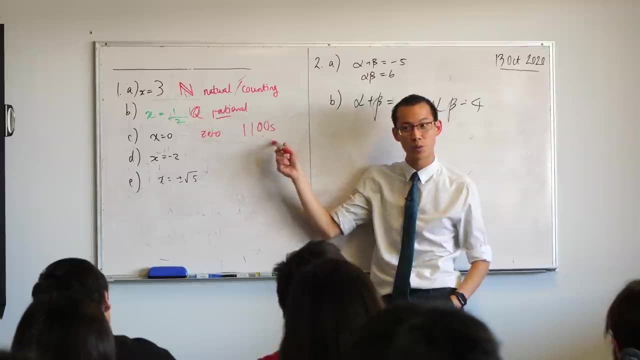 did a little bit better than that. From memory, it's the 1100s which is still like. oh, it's like at least we've got like a millennium, sort of. but still just think about how long we've been doing these and how long it took us to come. 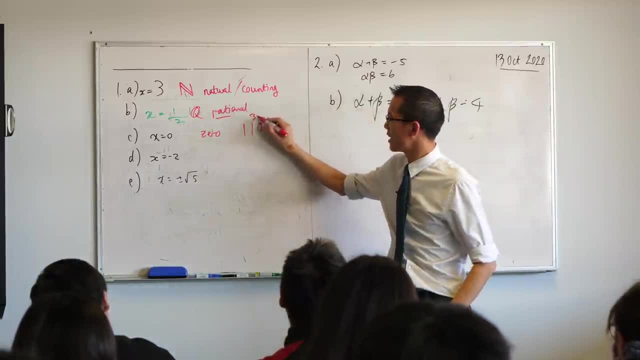 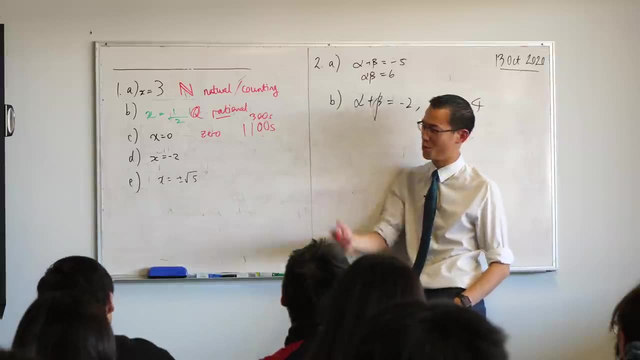 with this idea of zero. I should point out, by the way, Hindu and Hindu mathematicians in India beat us by several centuries. so I think it's really important that we recognise that Mathematics is a universal pursuit. Then we come down to these guys Back in year seven. we call these directed numbers, but 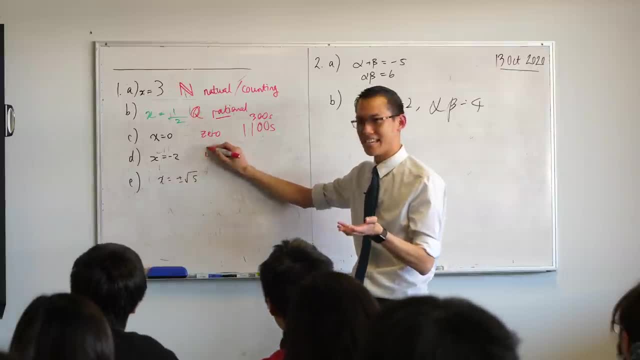 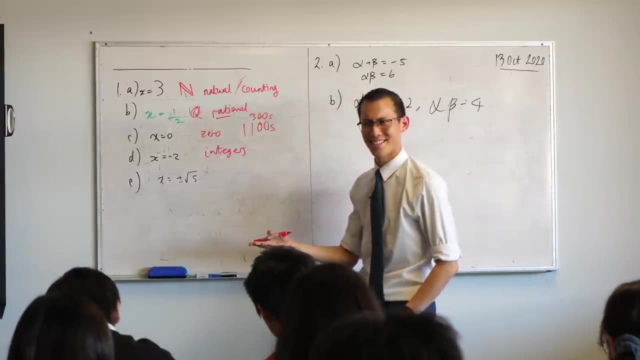 they have a more technical name starts with an I. anyone remember? These are the integers. again because we want to mess with you. the symbol for integers is not an I. Does anyone know what the symbol is? It's a Z. very good Again with. 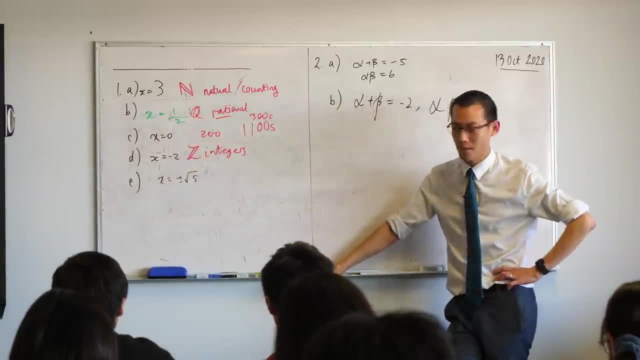 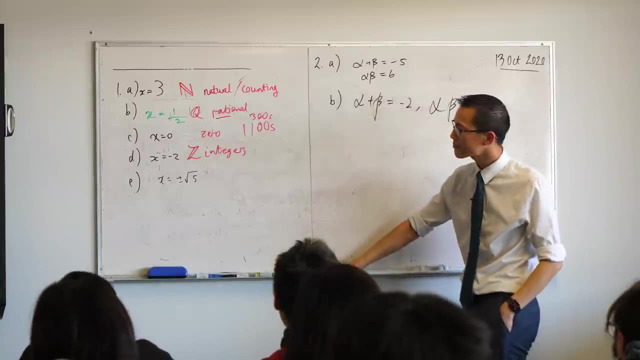 those two lines there A reference to the German mathematicians who did a lot of exploration in this field. Zahl Z-A-H-L is German for counting or counter. And then this last one down here doesn't belong to any of these sets. What do we? 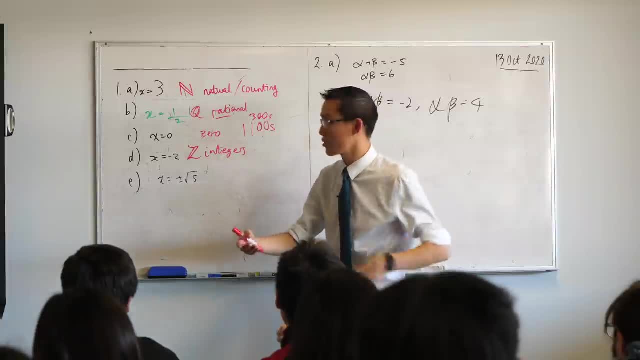 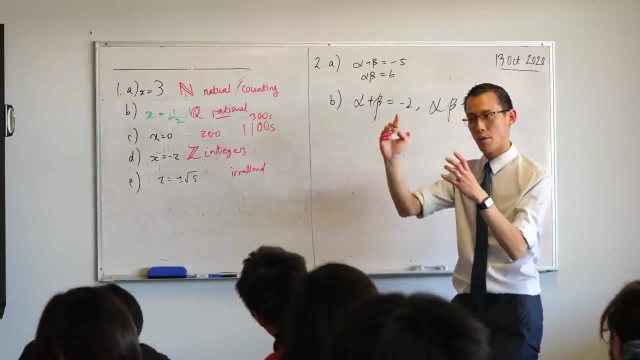 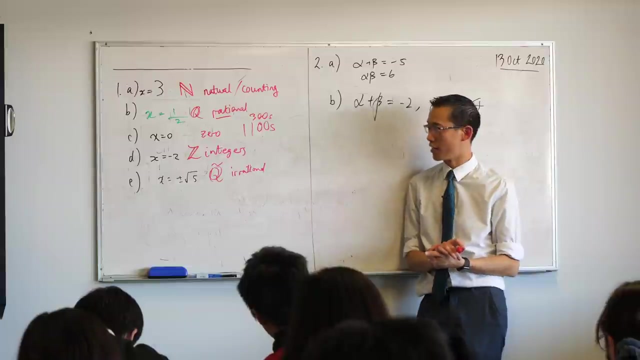 call this, We'll call it irrational, which is why irrational it's a name that means not one of these. We just take that symbol, the Q, and we pop a tilde over the top, which means not that, Not in the set of rational numbers. Now, the important thing I want to get. 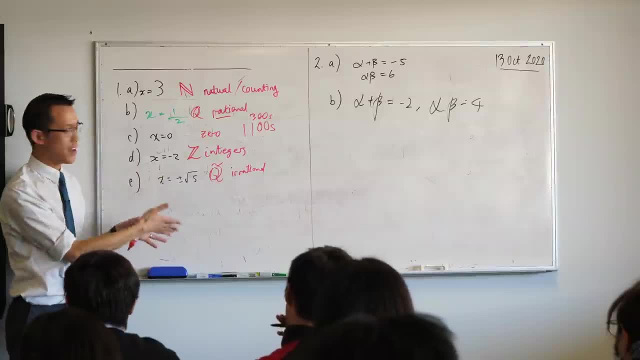 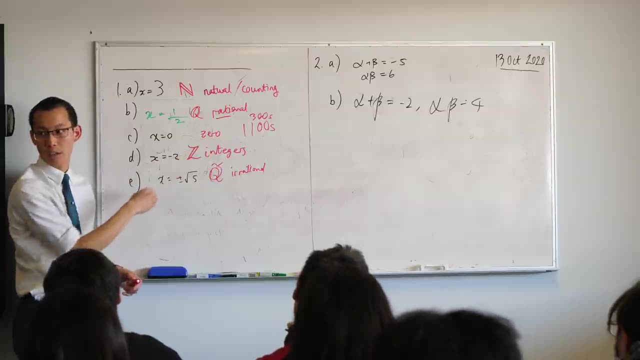 across to you as we looked through these is that each set of numbers it kind of breaks the rules of the previous set of numbers. If, for example, you have a look at part D, if you asked, like a five year old child, to subtract some numbers, they could do it. If you said, hey, what's? 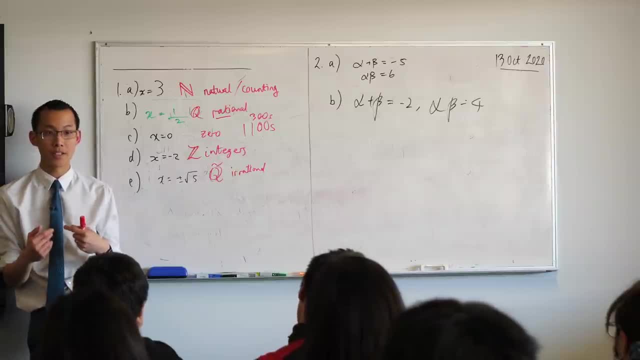 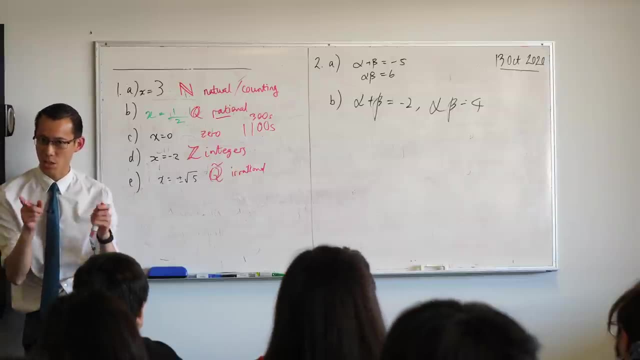 seven, take away three. They'd look at their fingers for a second and then they would repeat to you: four, no problems. But if you ask the same child, can you tell me what three take away seven is? do it the other way? they'd be like they'd get. 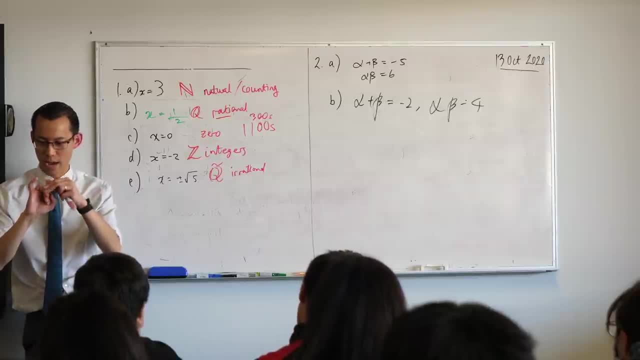 their fingers out and then they'd say, okay, well, here's my three. and then I start taking away to get to seven and I'm like, oh, you can't do it. No answer right Now. this was you many years ago. okay, but we came to realize. 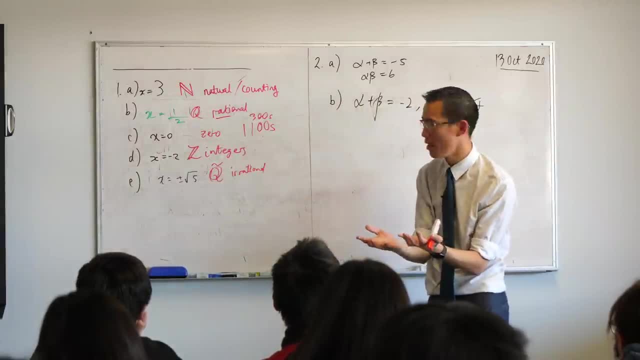 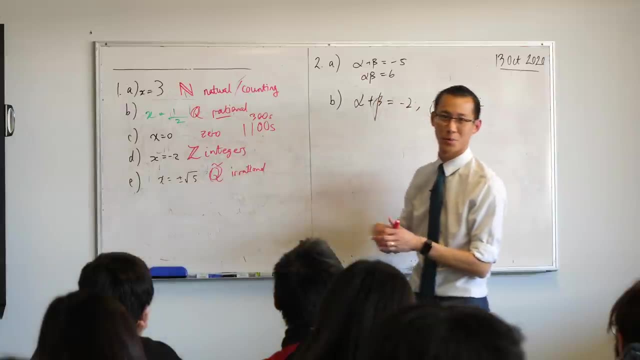 there's more to this than just the things that you can count. If we put direction on these numbers, that's actually really useful for things like temperature or debt. finance is actually where these were really, really useful. Now, this is kind of where we've gone. I should put on one more if you want to put. 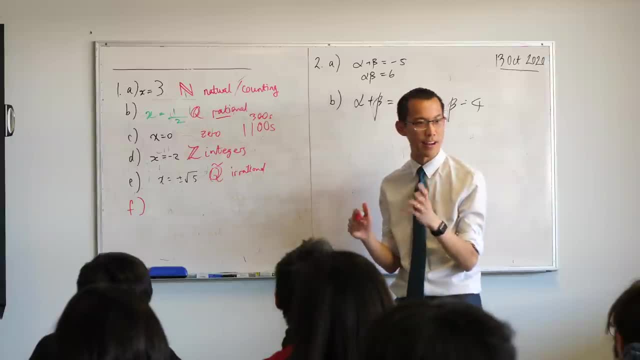 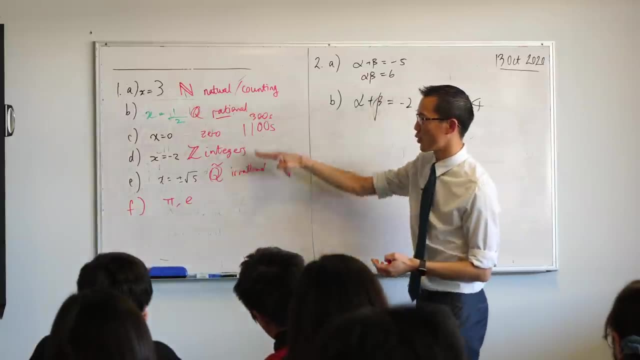 an F on here, for reasons that are actually really deep and profound. I couldn't write an equation that would do this, but you've got numbers like these guys right, Everything you just saw here. they're what we call the algebraic numbers, because you can form them with the rules of algebra Pi and E. you can't. 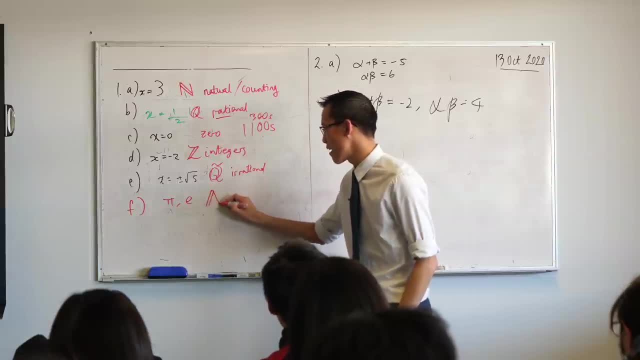 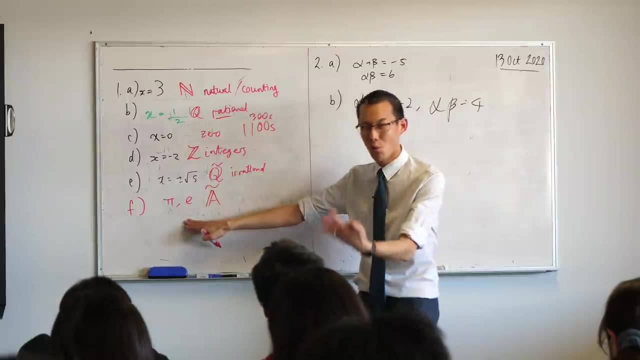 do that with those guys. so they're not algebraic. There's the A for algebraic numbers, so they're not algebraic. but because these numbers are so wicked and cool, we give them an even more special name. We call them- and this has to be one of the greatest names in- 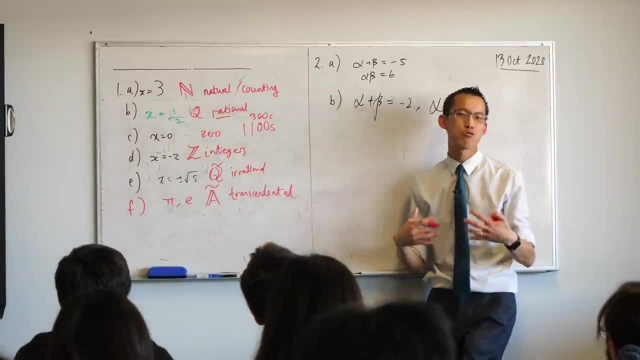 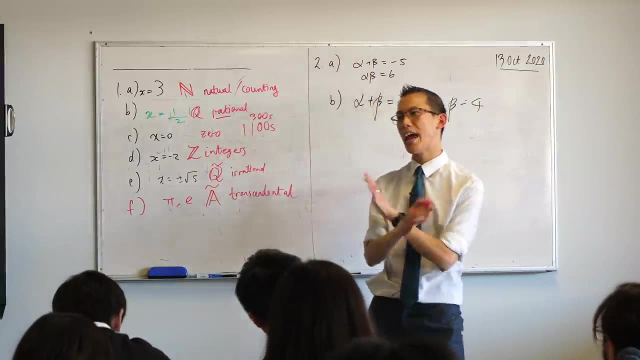 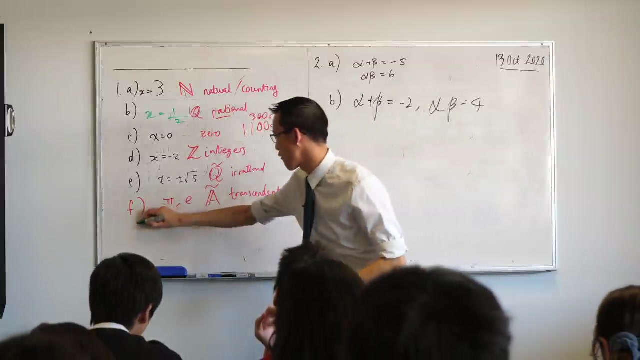 all of naming anything, really, we call these guys the transcendental numbers. okay, Now, if you take everything there, this is all the numbers you've ever had to do anything with in 12 years of schooling. All these guys as a big, happy family, they belong to one big sort of super set, if you like. and this one is: 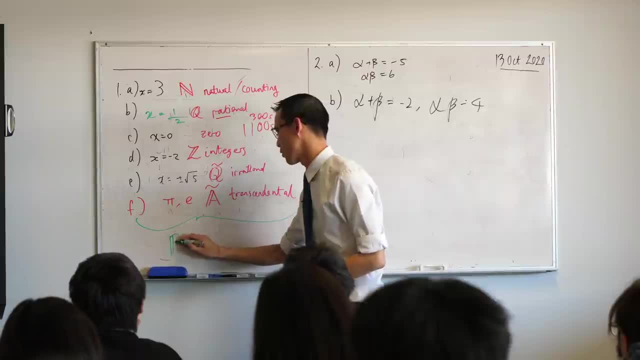 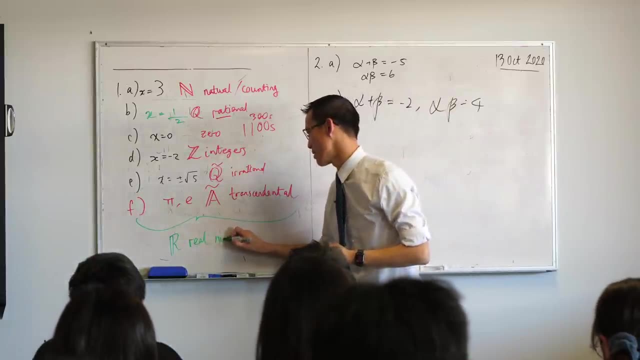 part of the reason why we don't use the R for this. This one does start with an R. It's a name maybe you've heard of. Does anyone know what these are called? The real numbers? Thank you, The real numbers. These guys are what you've been playing ball with. 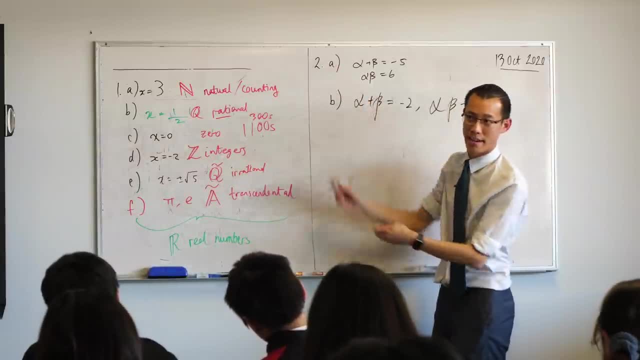 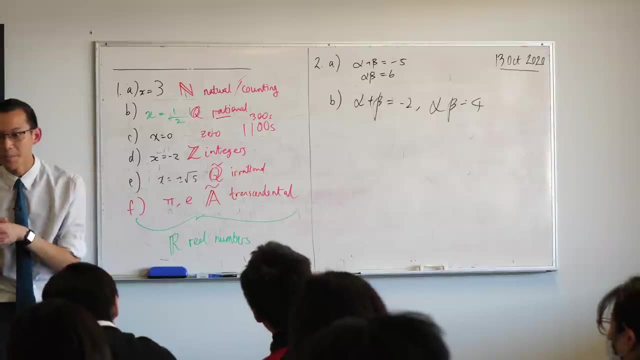 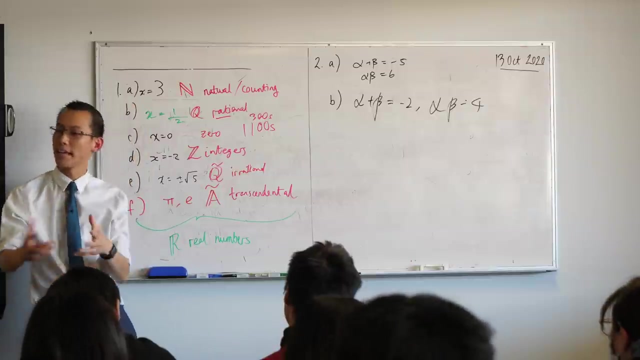 and, as you can see, they're inclusive of centuries of mathematical development. The real numbers, they're pretty cool. Just one teeny little problem, Yeah, question. I'm going to leave that very, very important distinction off of this discussion, mainly because I'm talking here about our progression through there. 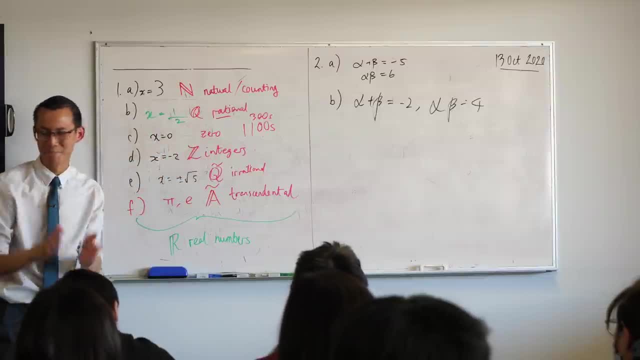 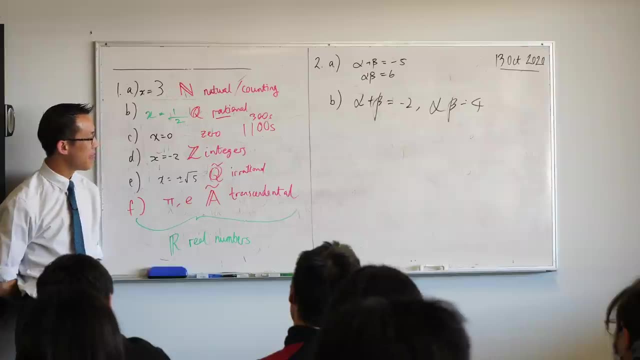 Does it include zero or not? You can see I delightfully dodged that question a little bit. We can have a discussion about that another time when we have more time. Good question though. So the real numbers, right, They include a lot of. 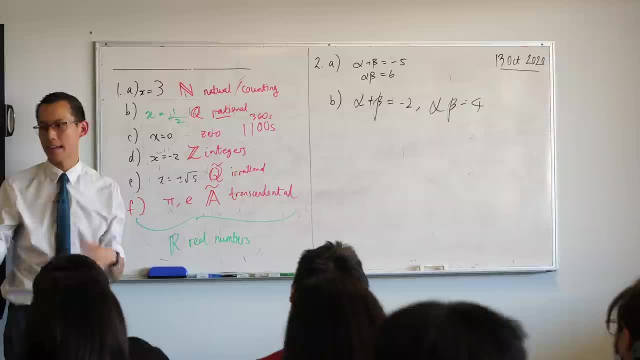 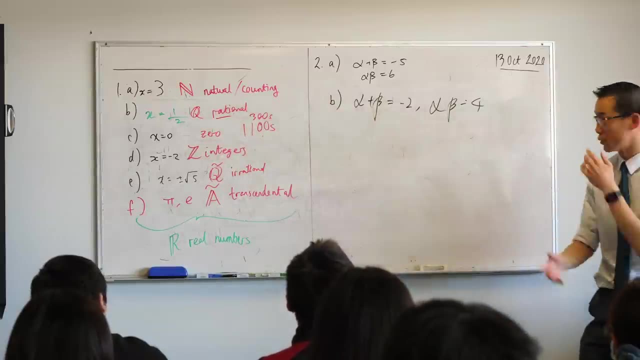 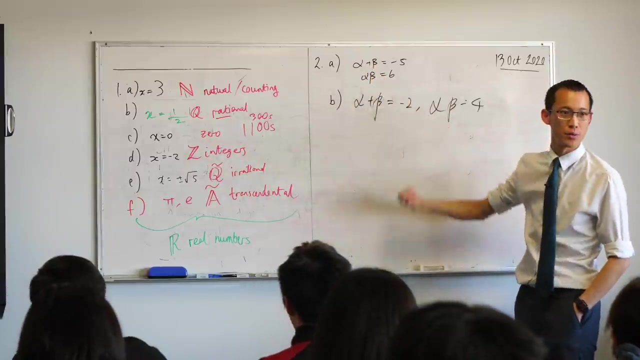 things, but there are signs in the mathematics. you've already done that. actually, there's more to the universe than this and my clue. there are many different clues, but my clue was in this pair of questions that I gave you here, right: Sum and product of roots. Sum and product of roots. Let's have a think about. 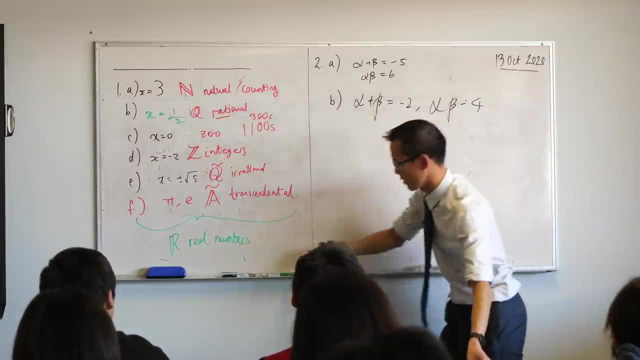 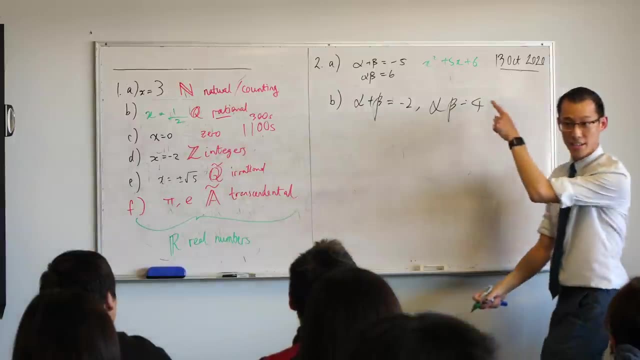 these guys for a second, Not this whiteboard marker. This was the equation I gave you, sorry, the expression I gave you for that sum and product of roots, and then, from memory, I think the expression was: this right, Is this right? Okay, great Now. 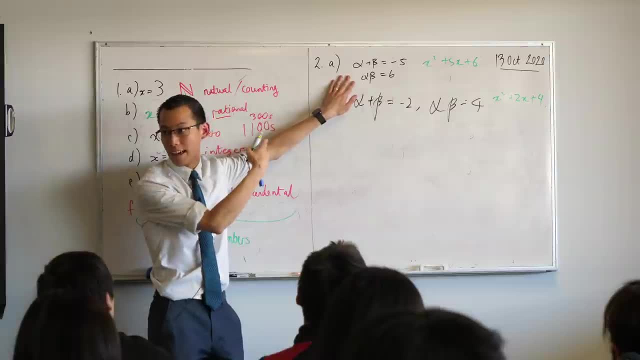 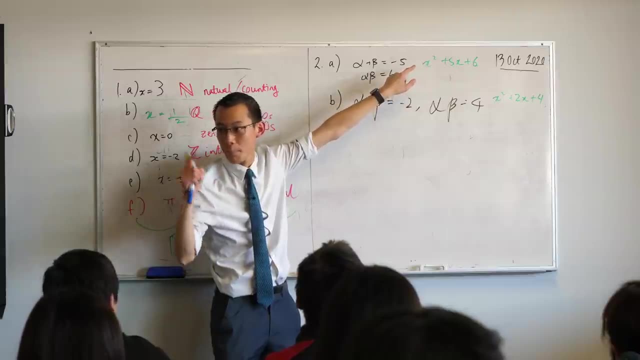 here's what I'd like you to do. I hope you went directly like this: whoever did this working did to alpha plus beta equals. how did you get that, by the way, It's what ratio is it? It's minus B on A. fantastic, and then for. 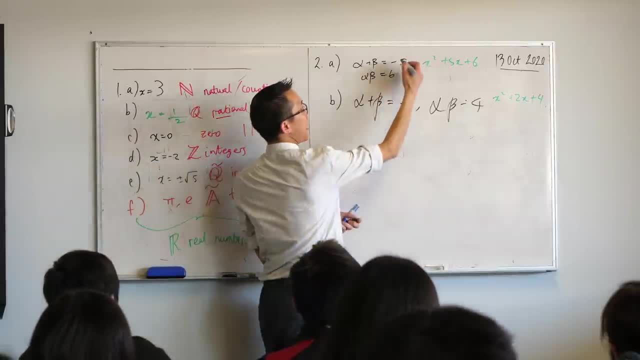 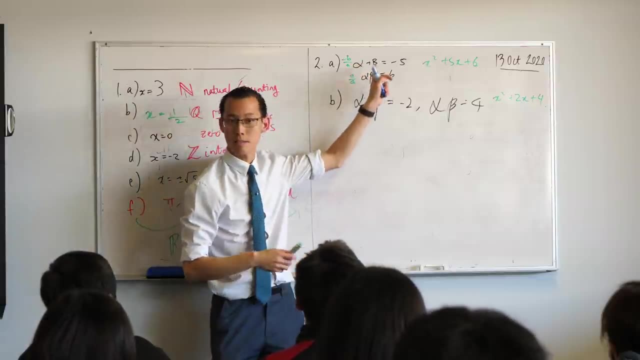 this: it's C on A. Okay, so we could go directly to those results without knowing- let's just write that here. without knowing what alpha and beta are, you can still work out what the independent sum and product are. right, Can you go ahead just for the sake of it. go ahead and solve this guy, right, You're? 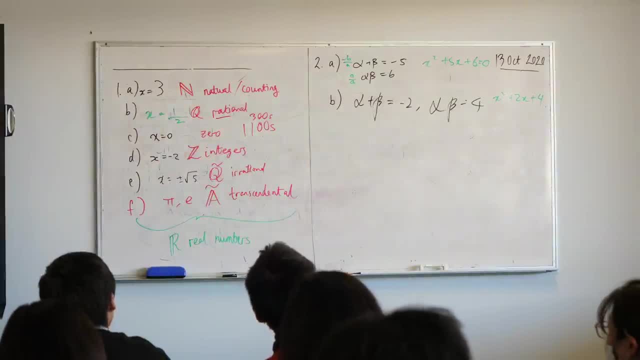 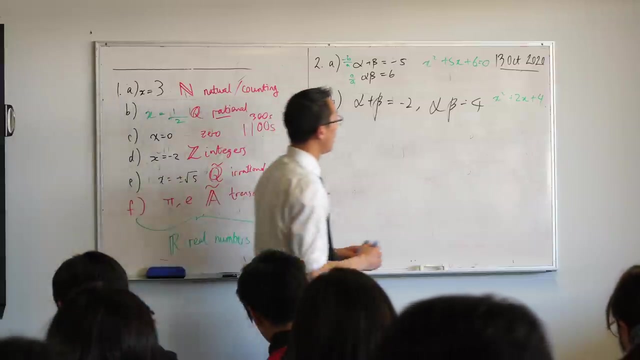 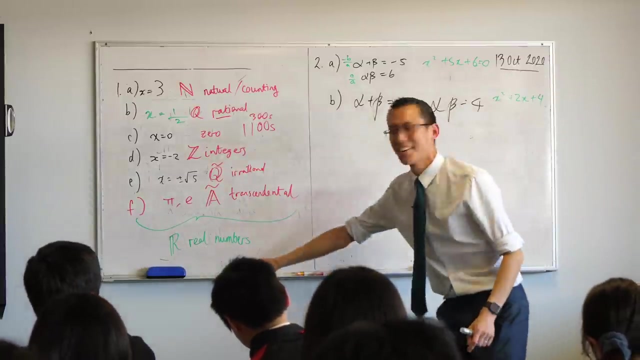 gonna get alpha and beta. Can you do that? Because I just need to wake up something on my screen for a second. Okay, that didn't take long, right? Go ahead and tell me: keep on picking up the same pen. go ahead and tell me- it doesn't matter which one's which, obviously- what are alpha and? 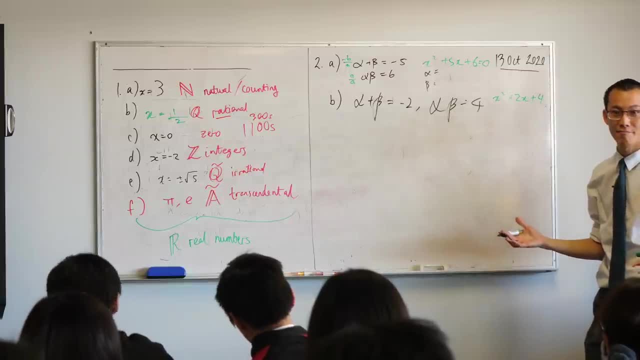 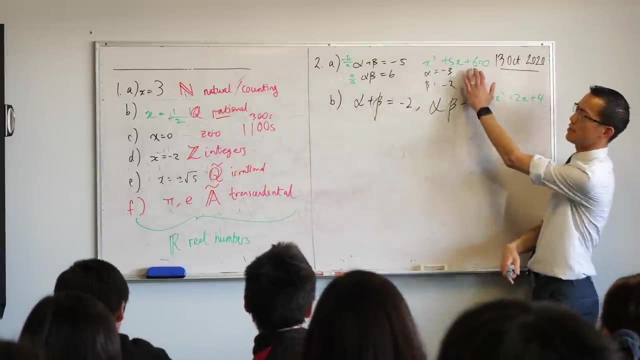 beta. what did you get? They gave three and Negative. Fantastic, and we could have interchanged them. that's fine. So we're like no big deal. of course they are negative three and negative two because you factorize this as x plus two, x plus three or whatever method you chose went. 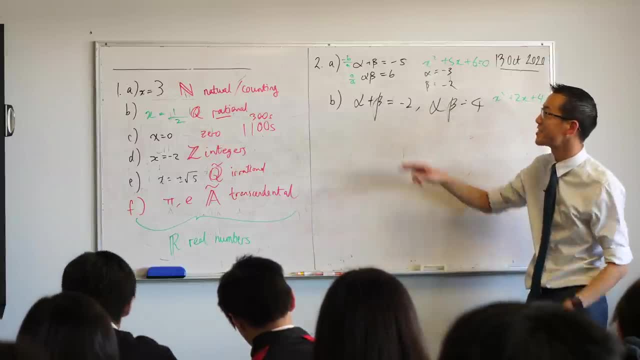 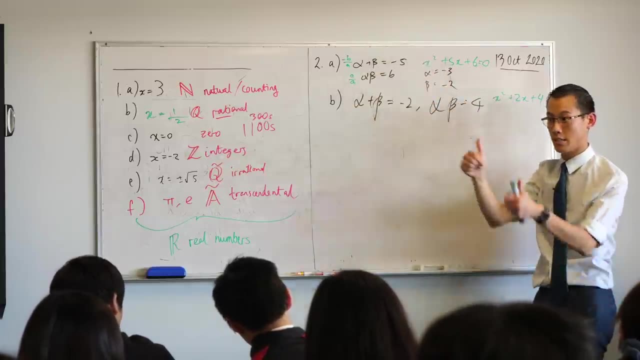 for the quadratic formula if you were particularly masochistic, and you can see, this confirms exactly what we saw here before. right, You add these two together, you get negative five. you multiply them, you get six. all good right, Except something. 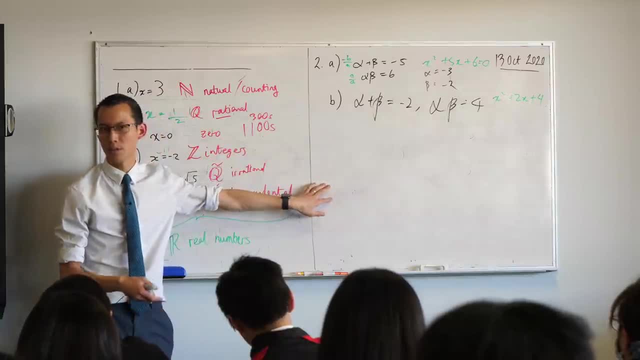 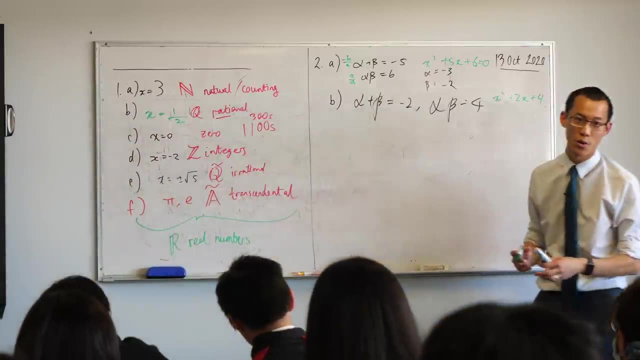 weird happens when you just have a look at this other seemingly harmless quadratic. and to illustrate this, we're gonna draw something You're gonna see. if, for those of you who are not in Mrs Lees' class, you might not know, we have an obsession. 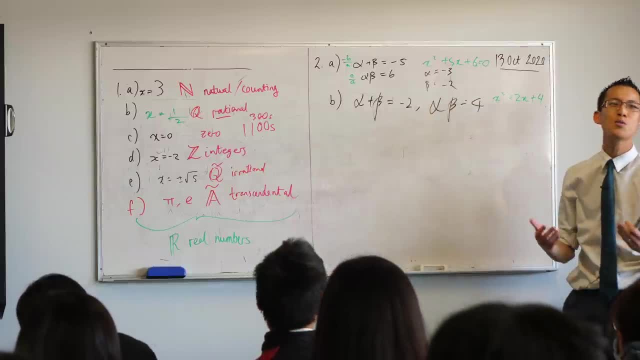 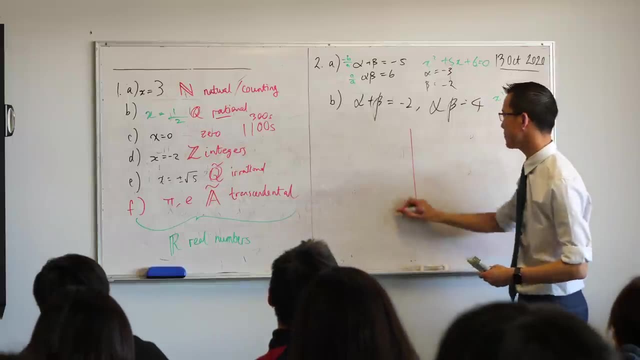 with graphing, even things you're like: why would you graph that? That doesn't say graph. we make you graph anyway because it's instructful, it helps you see things. So I want you to draw for me a set of axes, a Cartesian plane, and what I'd like to do is to take this quadratic. 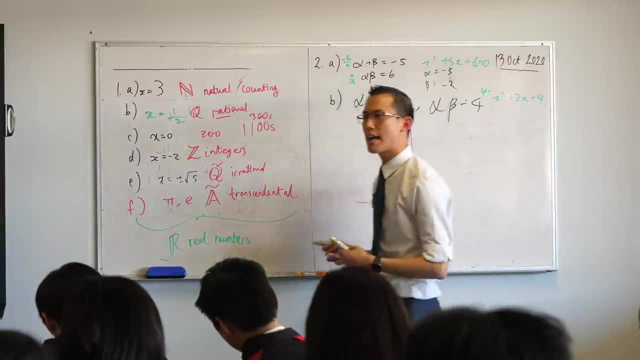 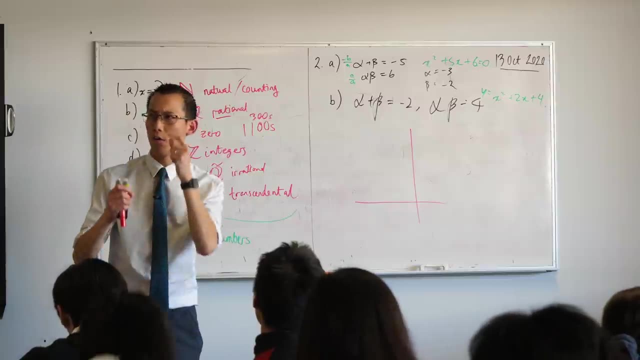 and to graph it. Now I'm gonna do it in a slightly unusual way. there are many ways to graph. y equals x squared plus two, x plus four, but I'm gonna try and call on the knowledge machine. Actually, it was around lockdown time actually when we were doing graphing. 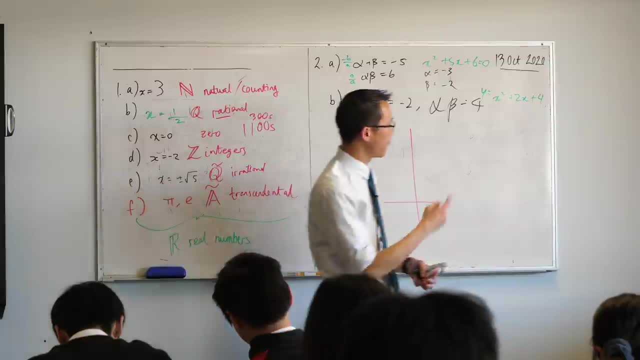 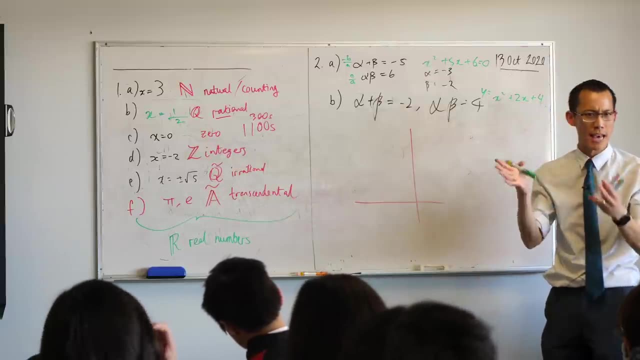 techniques in the advanced course, right, And functions like this we could think of in terms of transformations like stretching, dilation, shifts, that kind of thing. okay, So to do that, I'm gonna take this guy here and the first thing I'm gonna do is I'm going. 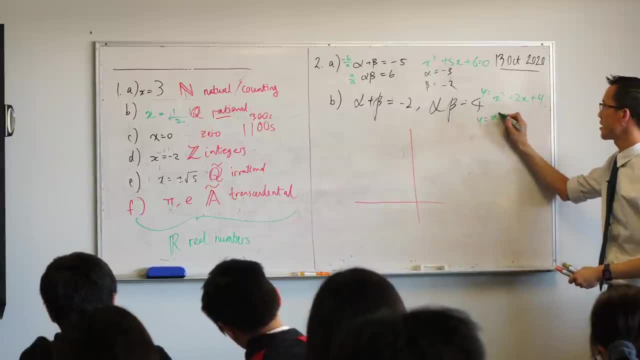 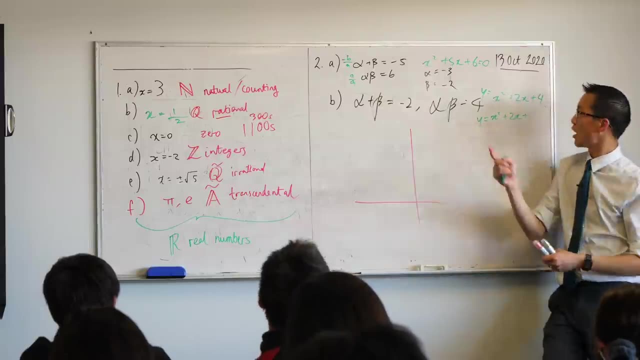 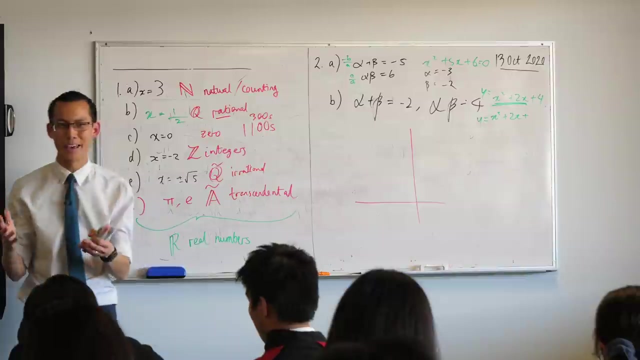 to separate out that four on the end there. I'm gonna separate it out into two different numbers, Two different numbers that are both inside four. that will come from completing the square on this guy. And you might think completing the square. that's a bit out of left field. why am I completing the square? This seems. 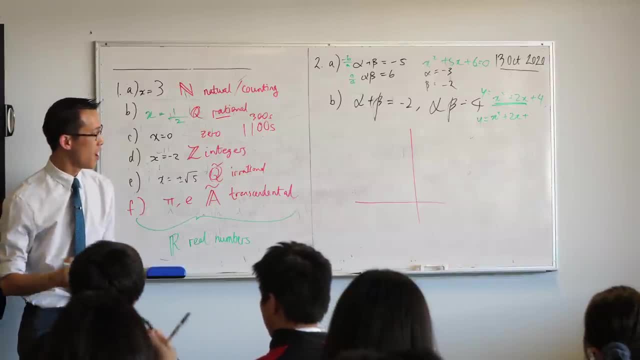 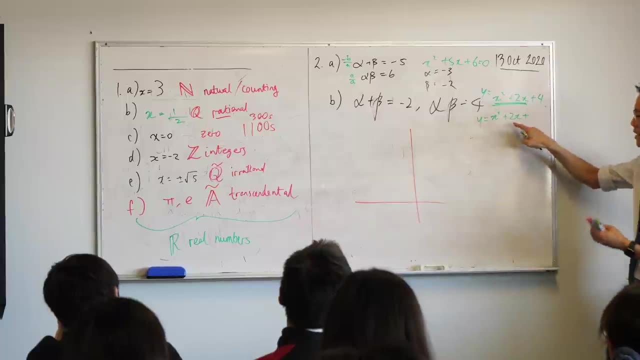 rather unnecessary. Stay with me, it will be useful in a second To complete the square. what do you add to x? squared plus two x, You add one. right, Because you take this coefficient here, you halve it and then you square it. In this case, you halve it, you get one. you. 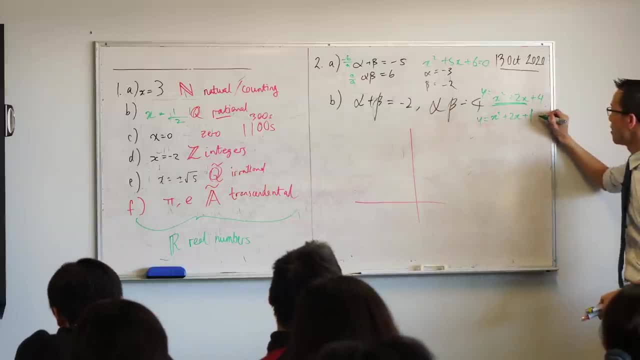 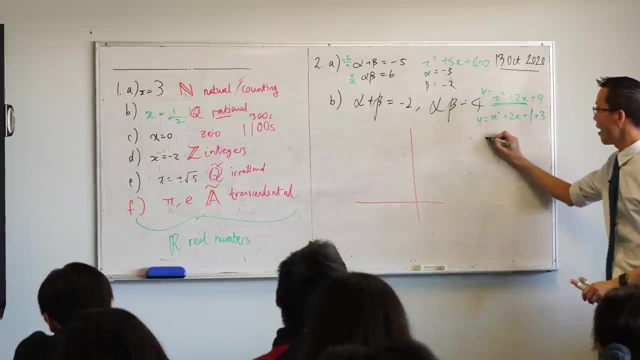 square it, you get one. So that's the one there. okay. That leaves, as part of that, four. That leaves a three On this side. okay, with that, One plus three is four, we're all good. The reason why we: 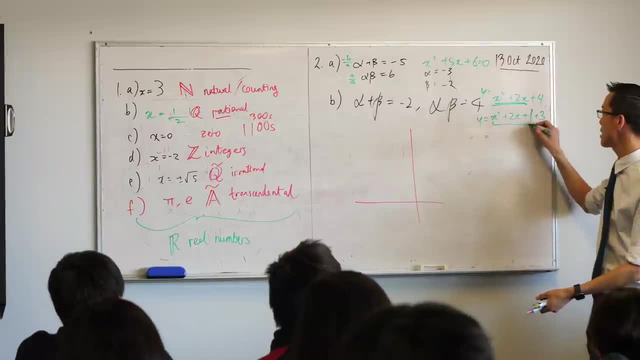 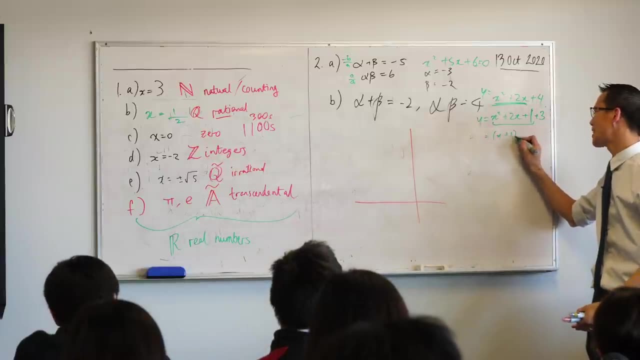 complete the square is. it's a useful way to factorize, right? So this thing here is a perfect square, namely x plus one all squared. I'm not that old, but you're gonna need to speak up a little bit for me, year 12, because, yeah, my hearing's not that great. So there's. 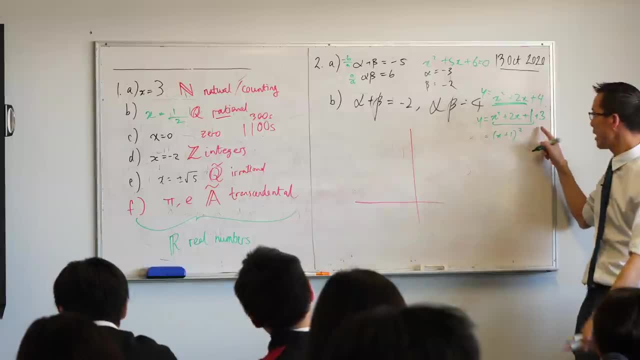 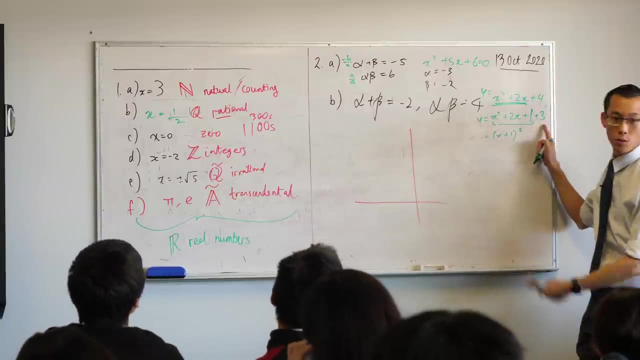 my perfect square. Now this plus three, I hope you can see it is actually go back to your graphing techniques. right? It's actually not interacting with the x. it's not about the vertical shift. It's really, though, it's on the right-hand side, it's really interacting. 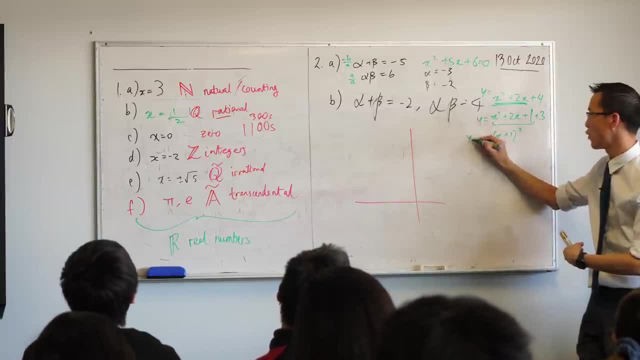 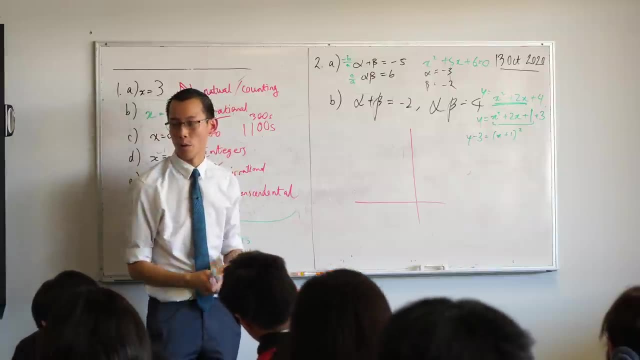 with the y. It's actually a vertical shift, So I'm gonna write it in this form: y minus three equals. Is that okay? Same deal: Three on that side, negative three on this side. okay, Why is this helpful? Why is this a good way to write this? Because when I come to 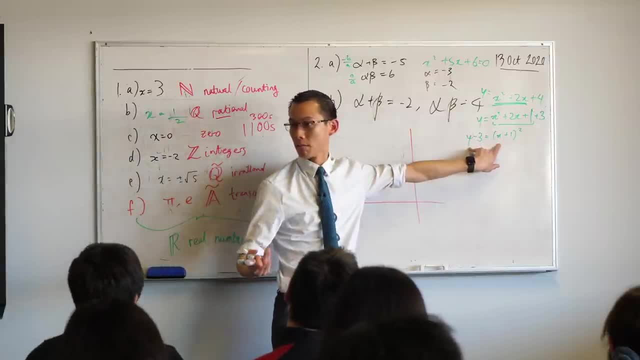 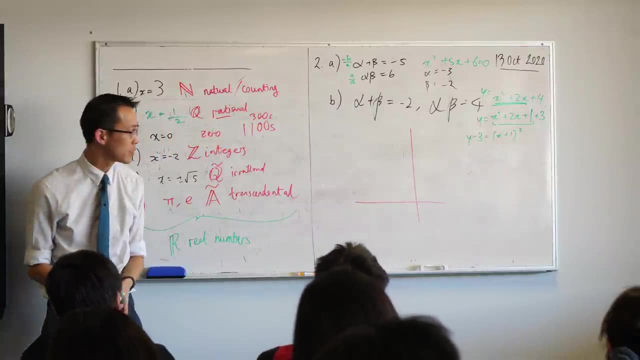 graph. I can now think of this as a regular old parabola like: y equals x, squared with two differences. What are the two differences? Those are the two numbers there. Can someone tell me one of them? What does the y minus three do?